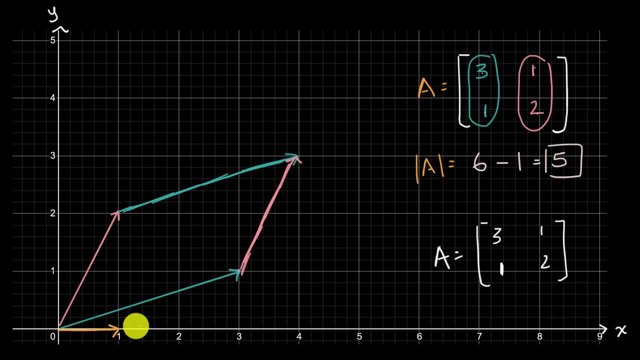 So, for example, I have this vector right over here, which is the vector one zero. We know that a transformation matrix. it says: all right, take that one zero vector and turn it into the three one vector. So turn that into that right over there. 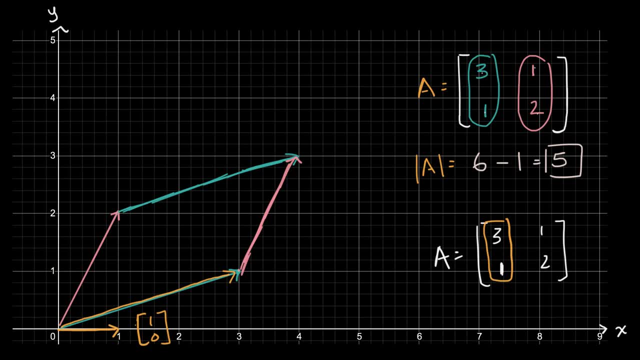 And we know we have the other or another unit vector. Let's call this this right over here is the zero. one vector goes zero in the X direction, one in the Y direction And the transformation matrix says, hey, turn that into the one, two vector. 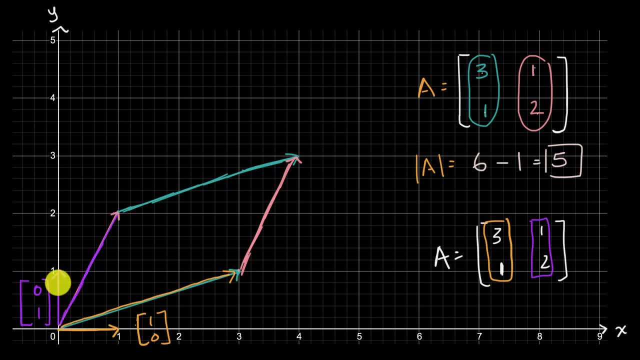 But then you could think about it, It's also not just transformation, transforming the individual vectors, It's also scaling up the area defined by the vectors. So the area defined by these two original- we could say unit- vectors, we could see it's one by one. 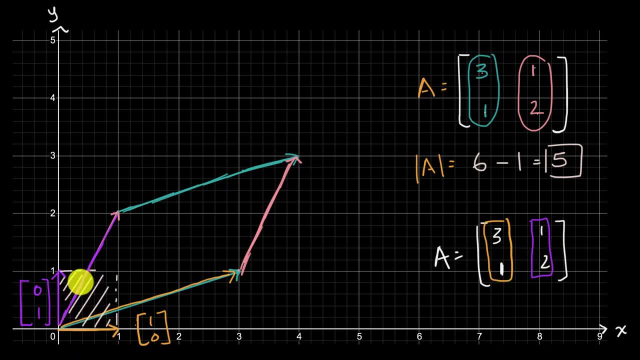 It's that area right over there. So this transformation is taking us from an area of one to an area of five. It's scaling it up by a factor of five. Now, that's reasonably interesting just for this one unit square, But because of that it'll actually scale up the area of any 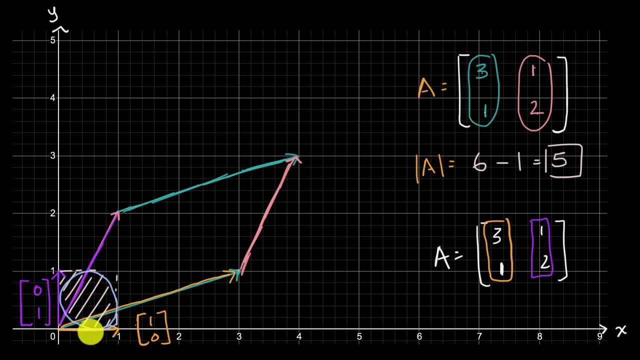 It'll actually scale up the area of any Figure. Let's say you had a figure like this. So this type of oval circle thing, it has some area. If you apply this transformation matrix, it will look something like this. I'm just approximating it. 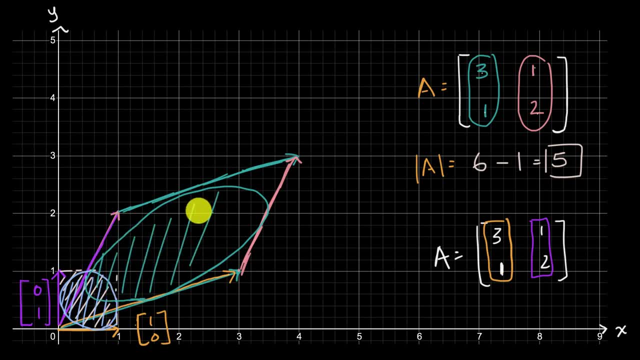 It would look something like that. So this will tell us that this bigger blob has five times the area of this original blue blob, because the bigger blob is the image. once we've transformed the smaller blob by this transformation matrix, by this transformation matrix, 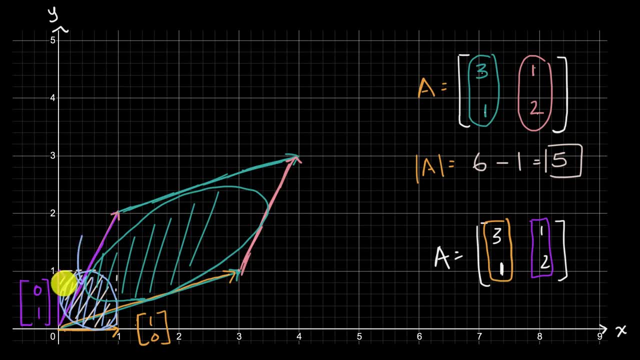 So this would tell you that the area of this smaller circle is, let's say, 0.6,. but then we were to apply the transformation and someone would ask you: what is the area of this bigger blob, which is the image of the smaller circle? 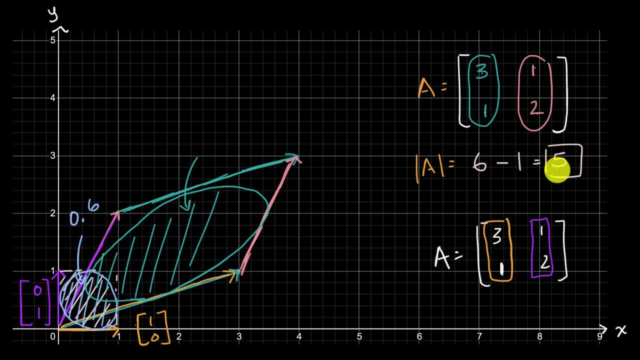 after the transformation. Well, you would take 0.6, multiply it by the absolute value of the determinant of the transformation matrix. You'd multiply it by five. So 0.6 times five would be three square units. So 0.6 times five would be three square units.